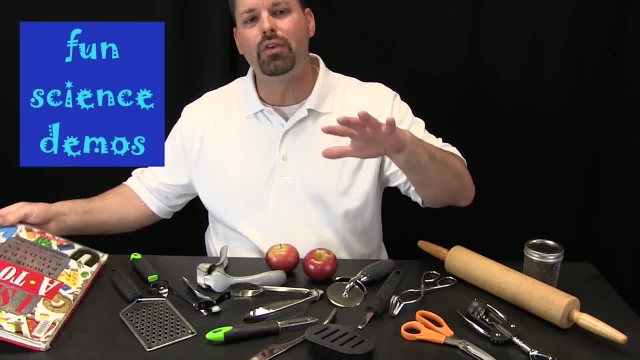 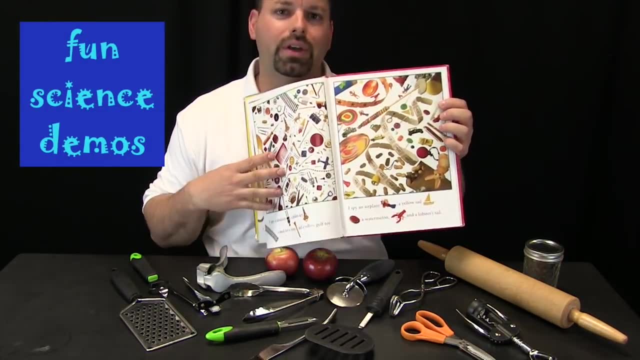 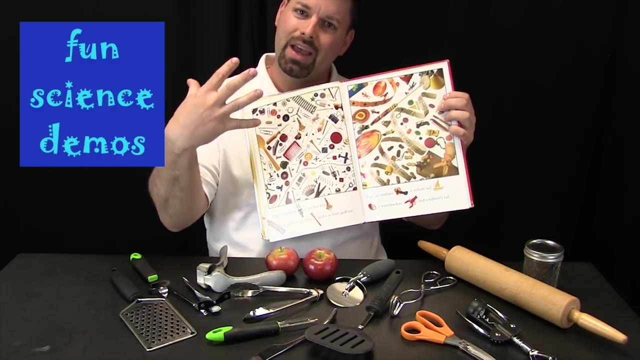 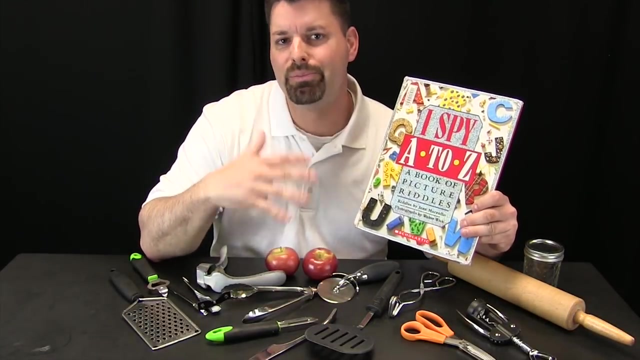 Hi, I am Jared. Welcome to Fun Science Demos. You know one of my favorite book series is the Eye Spy series. Let me open it up and take a look. What is so cool about this book is that they take random objects and just spread them on a page, and then you have to find certain objects hidden right in front of your eyes. You just have to search around. It is a great book series. The great thing about these books is that the objects that I am looking for are right there in front of me, but sometimes we do not see them. 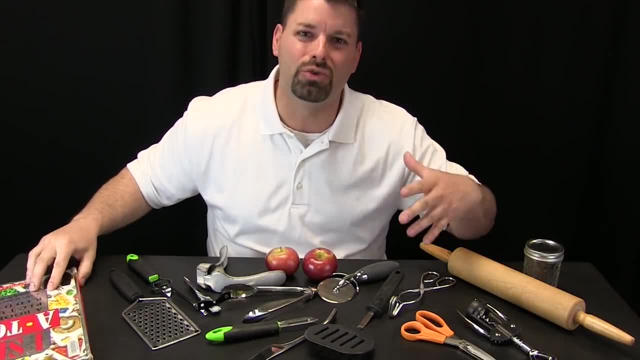 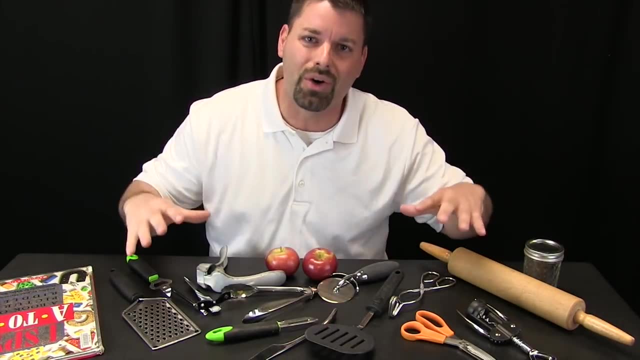 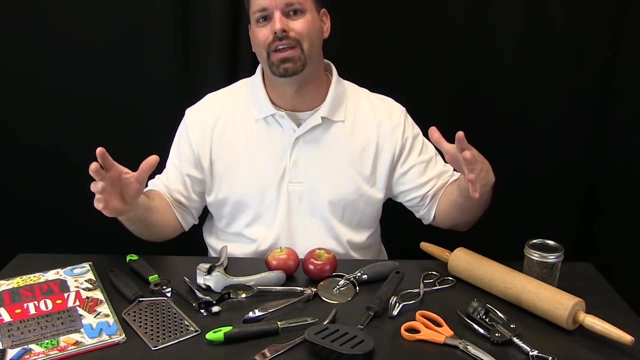 Well, here at Fun Science Demos, we think the same thing is true about science. Science is everywhere. Science is right there in front of our eyes, but sometimes we just do not see it. So here at Fun Science Demos, we came up with something we like to call Eye Try Science, to get us to really see the science that is right in front of us. 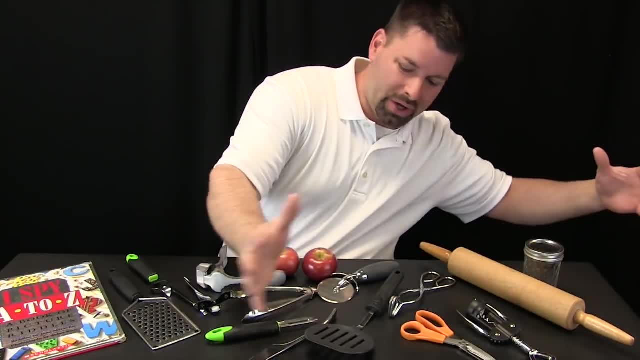 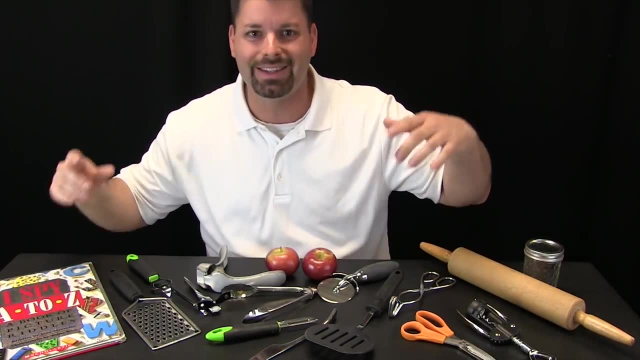 So I went into my kitchen and I just took a whole bunch of random things, all these different objects right in front of us, And we are going to see if we can try to find the science in these things, specifically the science of simple machines. 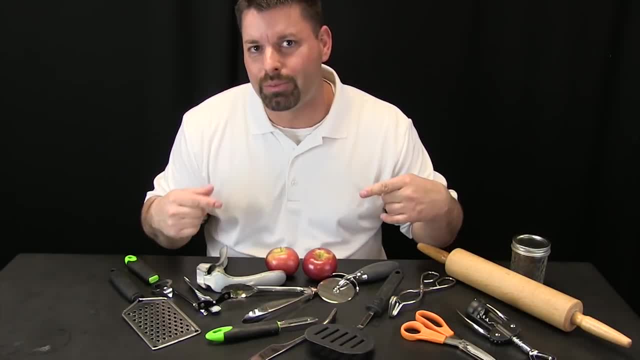 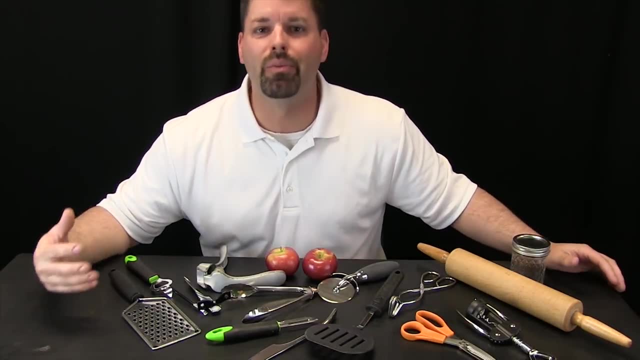 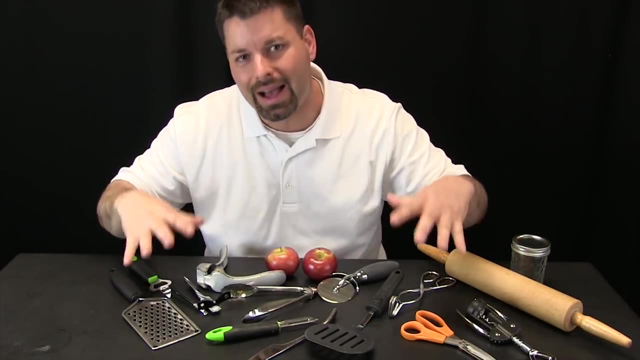 In some of our other videos we have actually talked about some of those simple machines, Some things like a lever or an inclined plane or a wedge and a wheel and axle, And we have also talked about pulleys. Well, today we are going to try to find some of those simple machines in these everyday objects by trying them out. 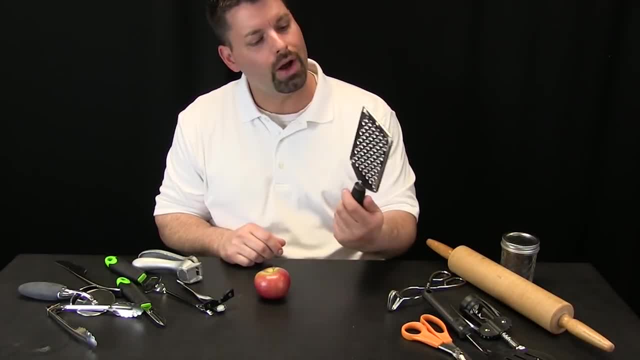 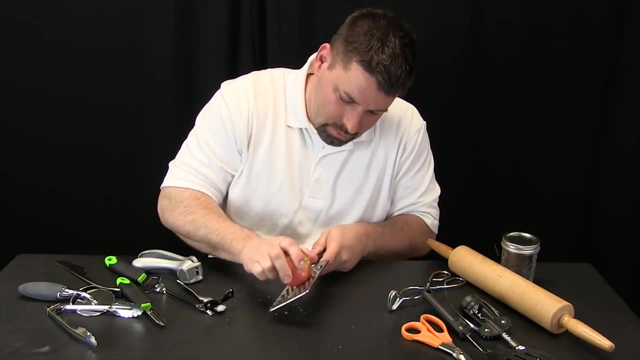 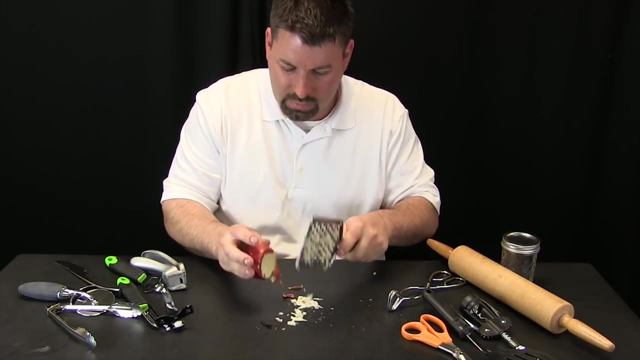 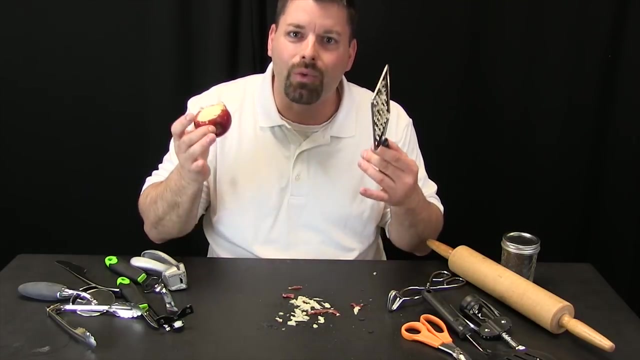 Eye, Try Science. So let us start by trying this grater and see what happens when I try to run the apple over it. Here we go. Now I have made a mess, but making a mess is part of science. But what do we spy? What do we see after we have tried this? 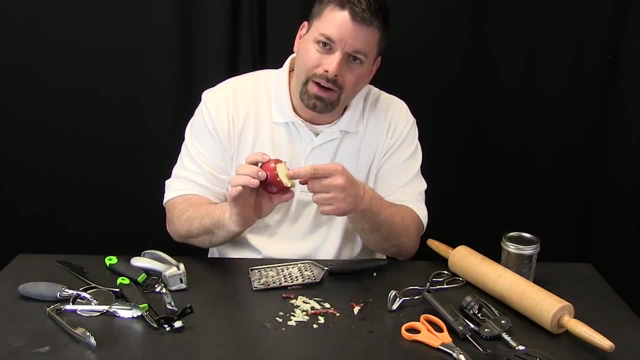 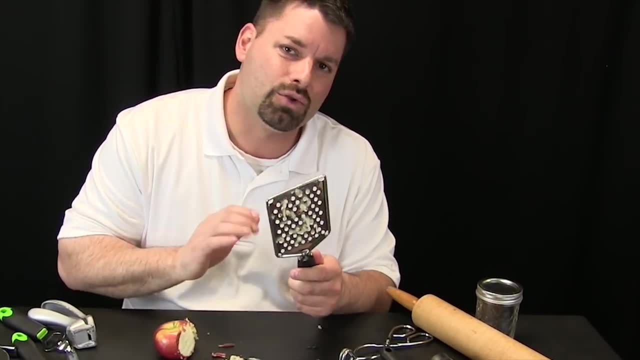 Well, I see that little parts of the apple were actually removed. Well, I see that little parts of the apple were actually removed. Well, I see that little parts of the apple were actually removed From the other part of the apple. To me, after trying this, I think that this grater is actually a wedge. 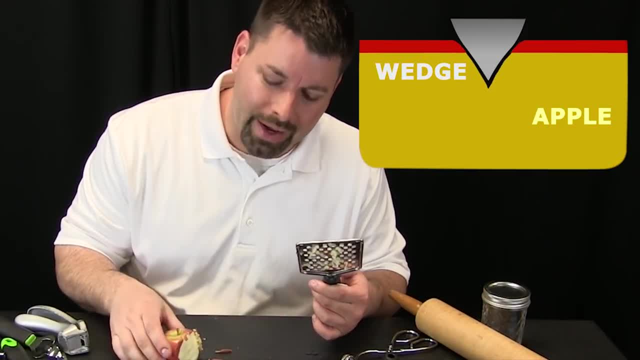 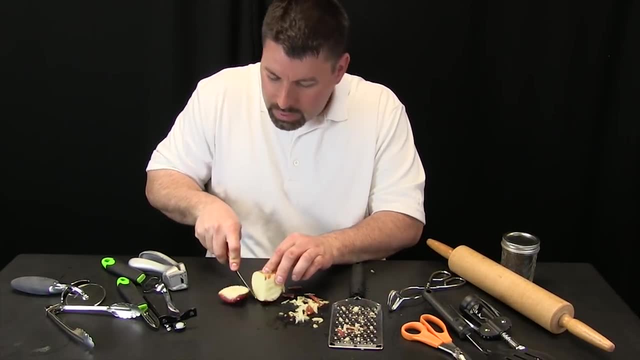 So this grater is a simple machine. It is a wedge that separates this apple into smaller slices. Next, I am going to try this knife. Next, I am going to try this knife. And what do you know? This knife does a great job separating this apple also into smaller pieces. 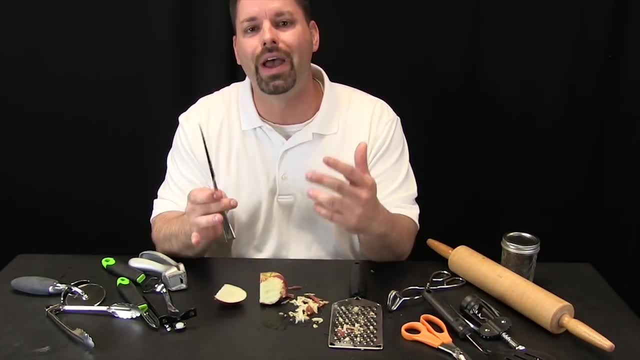 So what do you think this knife is? What kind of simple machine. I think it is a wedge. So now I have a chunk of apple And I want to see if I can try to get this into a smaller piece of apple. I am going to try this. 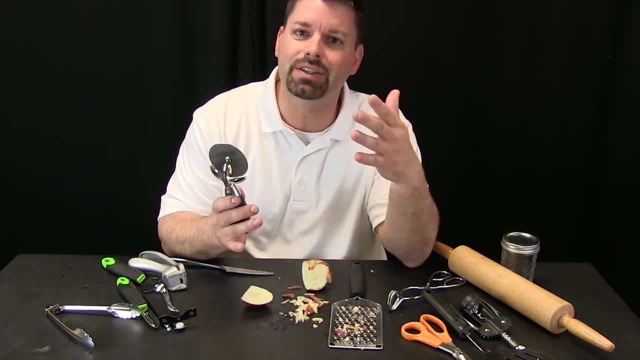 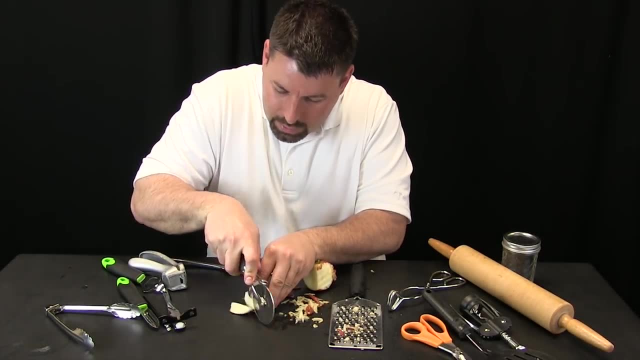 Now, I know a lot of people normally will use this to cut pizza into smaller pieces, But I want to use this to see if I can cut my apple, So let us give it a try. Wow, that made the cutting so much easier. 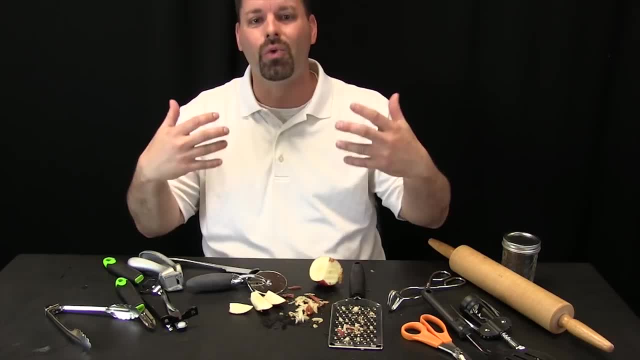 Well, that is exactly what simple machines do. They make our work easier, And you can see I have separated this apple into smaller pieces. And you can see I have separated this apple into smaller pieces, So that must mean this is a wedge. 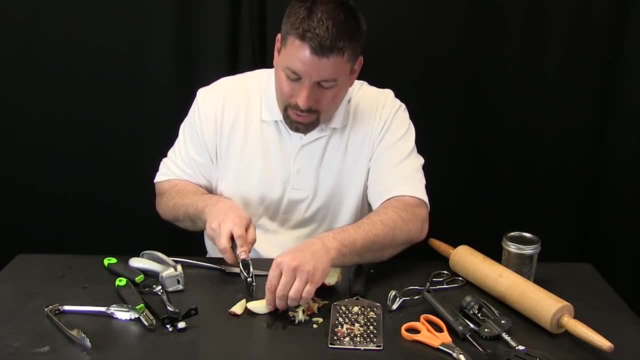 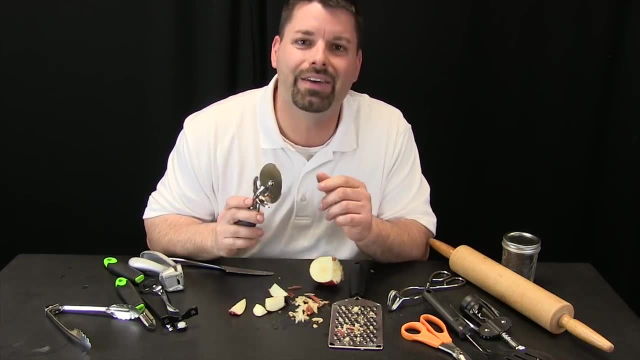 But did you notice something else? I pushed it. Watch carefully, This rolled, It spins. What kind of simple machine do you think that is? What kind of simple machine do you think that is? So we have zoomed in so you can see our wheel spinning. 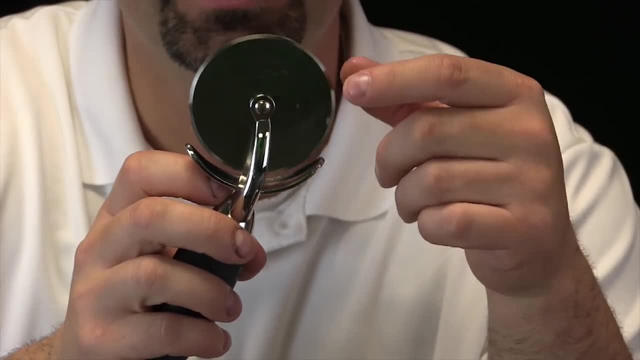 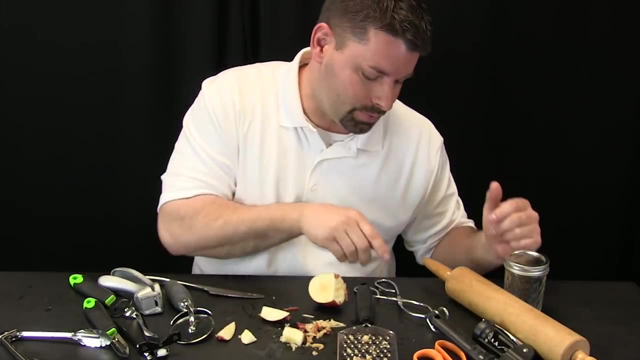 And I just gave you a clue. This simple machine is a wheel and axle. This simple machine is a wheel and axle. So now I have a small pile of apples, But I do not want to get my hands messy picking it up, So what can I use? 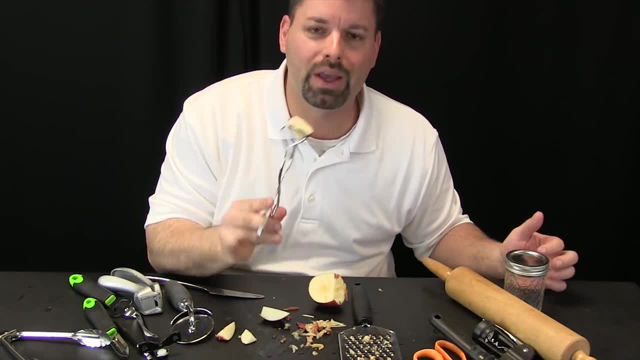 I can use my trusty tongs. I can reach down and pick up a chunk of apple. What kind of simple machine do you think these tongs are? What kind of simple machine do you think these tongs are? These tongs are a lever. 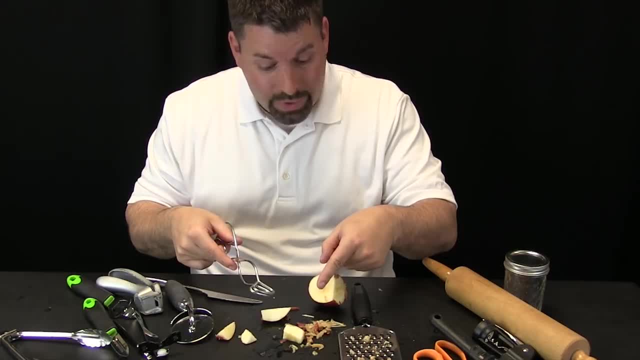 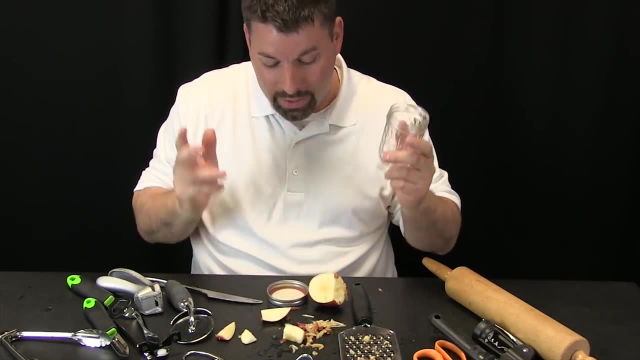 These tongs are a lever And they are going to help me put all of this apple, clean it up and put it into this jar. So here we go, Unscrew the lid And wait a second. Think about what I just did. 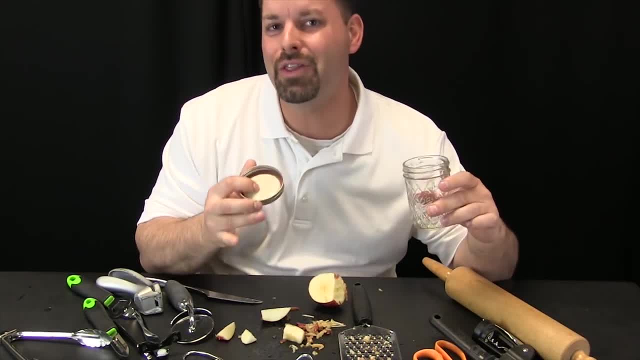 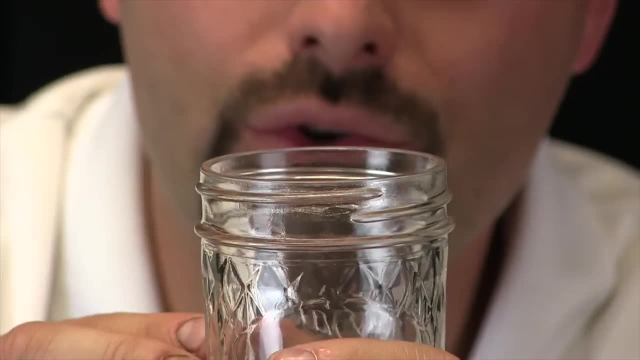 I unscrewed the lid. I have just found another simple machine at work. I have just found another simple machine at work. What kind of simple machine do you think this lid is? What kind of simple machine do you think this lid is? We have zoomed in so you can take a closer look at our jar. 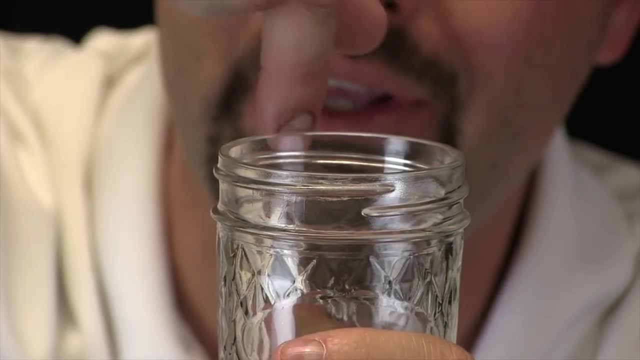 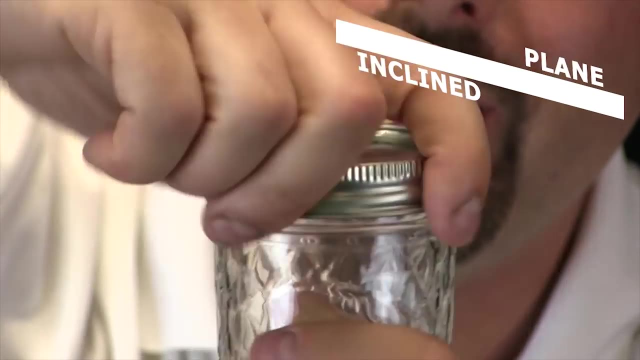 And I want you to look at this glass line. It slowly goes up as it wraps around the jar. It slowly goes up as it wraps around the jar. That is actually an inclined plane, And what that allows me to do is to screw the lid on.